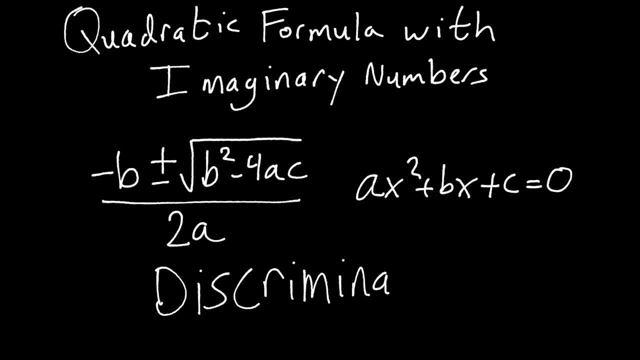 The discriminant is something called the discriminant, And the discriminant is this stuff that I am circling in purple. The discriminant, while to some people may not be vital to solving the equation, it can give you a heads up as to how many real or non real solutions you are going to have. So we 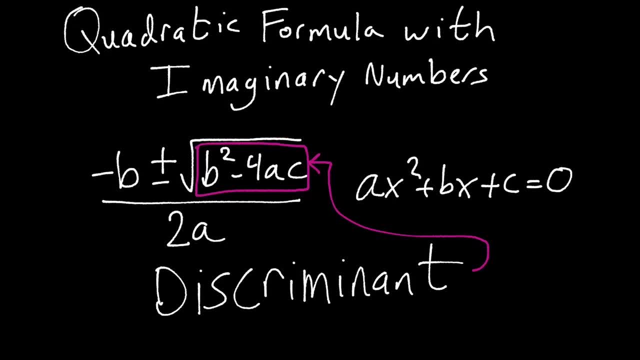 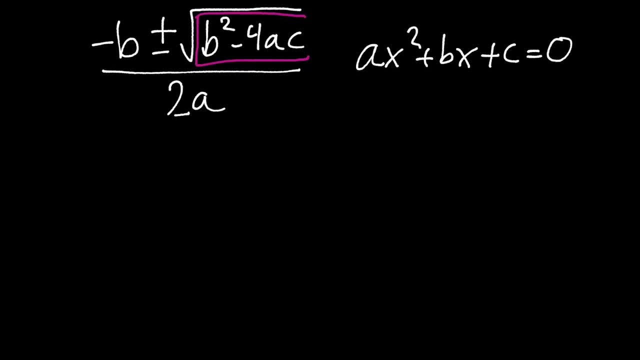 are going to start by using that discriminant, and then we're going to solve a couple problems together. Let's begin Alright. so our first example is going to be: x squared minus 2x plus 10 equals zero and, as you hopefully notice, this matches our quadratic formula example up here. 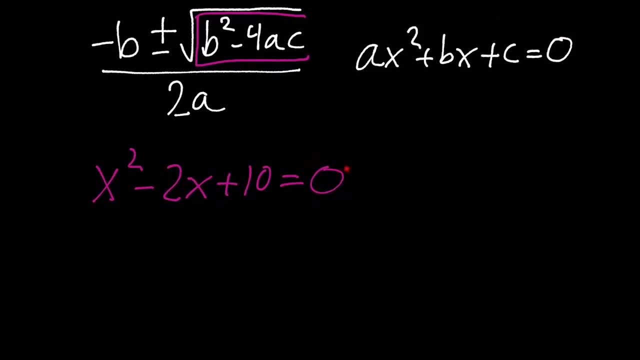 because we have an x squared term and we are equal to zero. So we should label our a, our b and our c. a is over here and since there's nothing in front of the x-squared term, it's actually 1, b is 2, sorry. 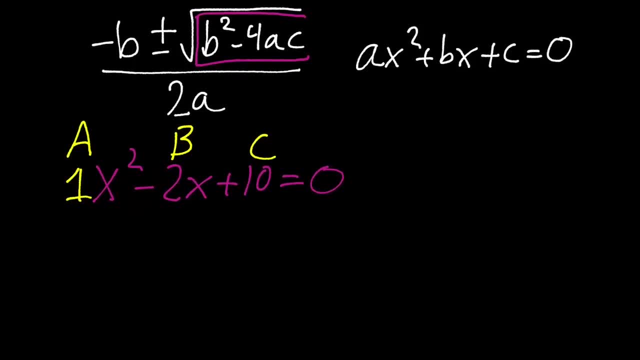 negative 2, because don't forget that you have a negative sign there, and c is 10. now, before we plug everything into this equation, we need to take a look and find the discriminant which I've left highlighted up top there. so we just want b squared minus 4ac. 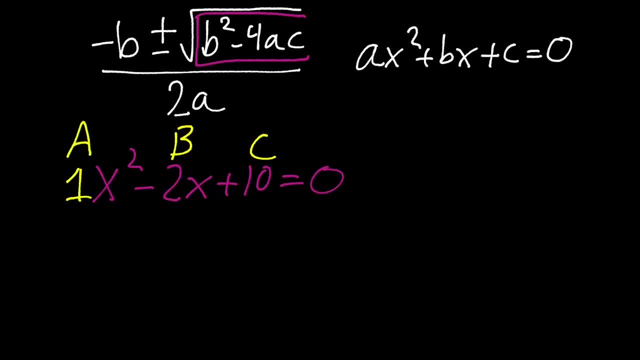 well, b is negative 2, so I have negative 2 squared minus 4 times a is 1 times c, which is 10, and by solving this it can tell us how many solutions we are going to have with our, with our quadratic equation, it could be two real solutions. 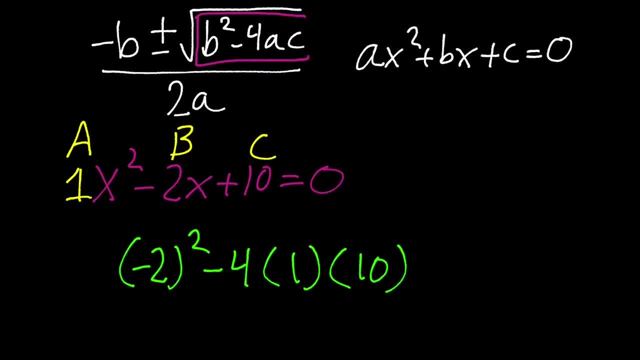 it could be one real solution or it could be no real solutions but two non-real solutions, which is going to be the purpose of this video. so you can probably guess we're gonna have some non-real solutions when I solve this. negative 2 squared is 4. 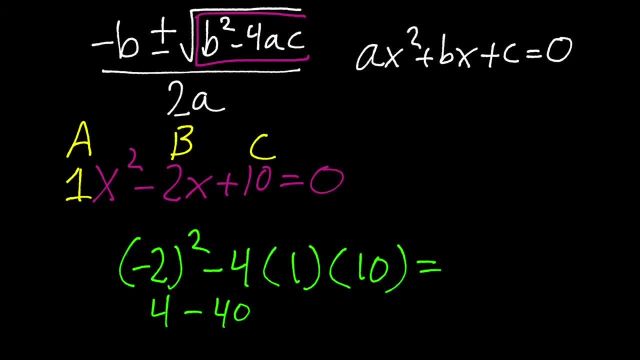 minus 40. 4 times 1 times 10 is 40, so this gives me negative 36. now, the fact that this is negative tells me that I am going to have non-real solutions, and a quick way to helpfully remember this is: let me move this up real quick. 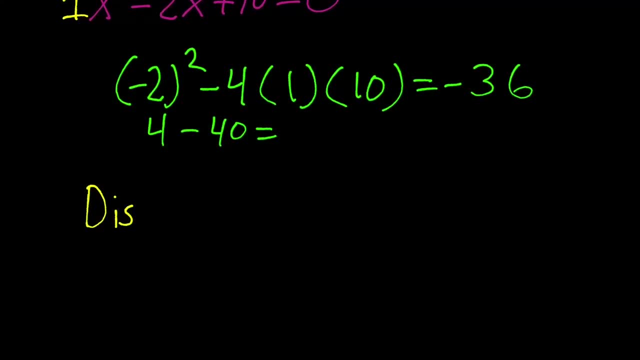 if the discriminant- which I'm just going to abbreviate DISC- is greater than 0, meaning positive, you get two real solutions. if the discriminant is equal to 0, you get one real solution, and if the discriminant is less than 0, you get 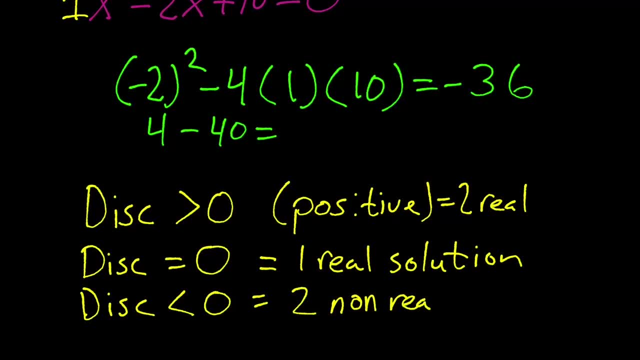 two non-real solutions, which is what we just ran into. we're gonna have two non-real solutions here because of that square or, sorry, because of that negative 36. so now that we've got that, let's figure out what these non-real solutions are. so I'll move this back up. we already know. 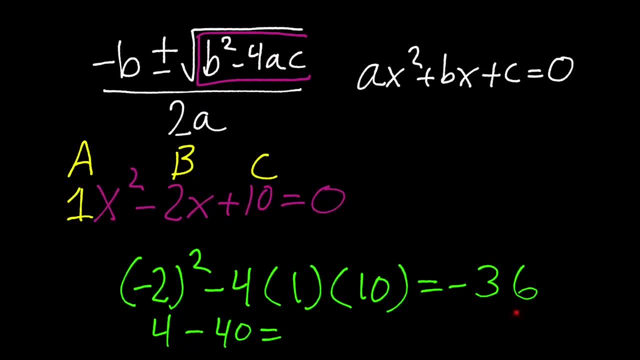 that everything on the inside here is negative 36, so I don't have to plug everything back in using the big formula. I already know this is negative 36, so let me erase and we can start getting our two non-real solutions. we'll start off with the opposite of B. 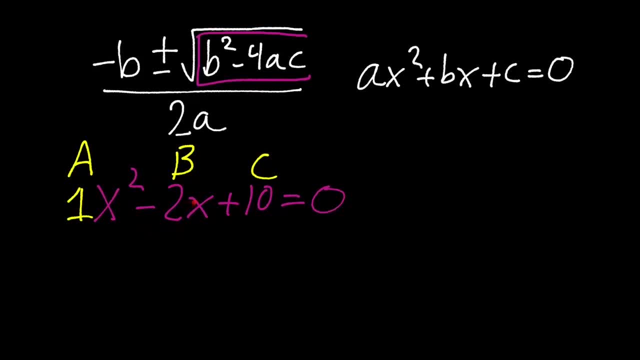 since B is negative 2, the opposite of B is positive 2 plus or minus. the square root of that discriminant, which we said was negative 36, all over 2 times a, and a is 1, so 2 times 1. now, if I try to solve this, 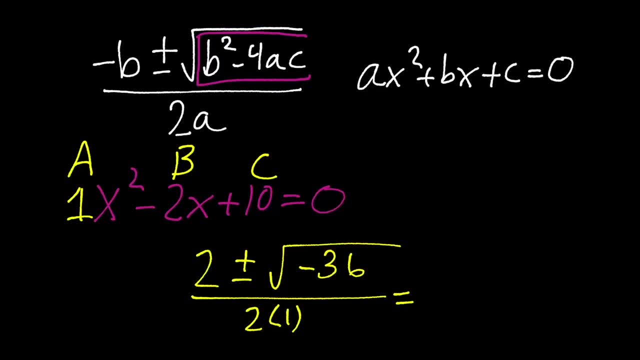 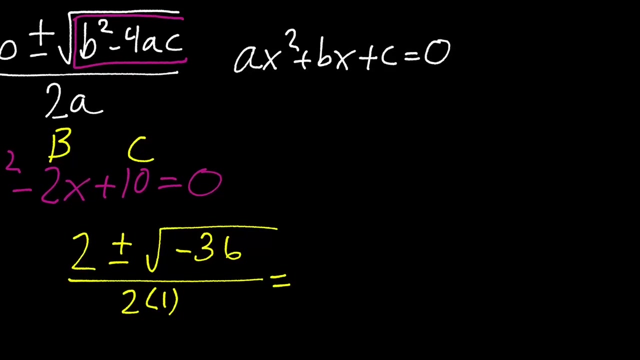 we notice, hopefully we notice. anyway, my discriminant is negative 36. I'm gonna have to take the square root of a negative number which we talked about in my last video, but this is also a perfect square. that's pretty nice. so if I want to slide this over here, the square root of negative 36. 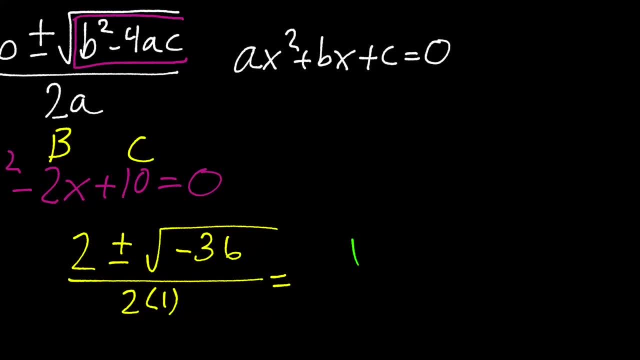 is the same thing as the square root of negative 1 times the square root of 36. this is a perfect square. so, just like in the previous video, this can become just 6. this becomes I. so this simplifies down to not just the square root of 36, but instead. 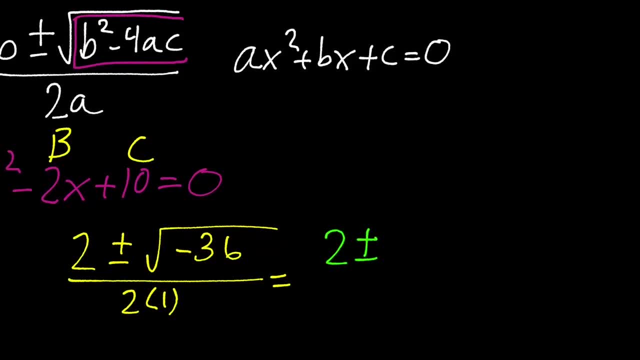 we get 2 plus or minus 6i, all over 2, and you could leave it in the next step if you want to this form. but if we want to be a good mathematician, since both terms up top are divisible by 2, 2 divided by 2 is 1, 6 divided by 2 is 3, we can change this. 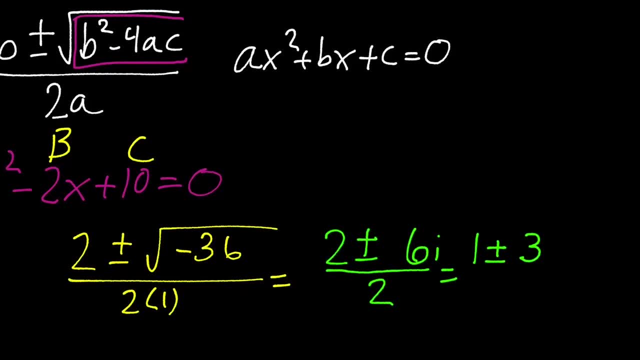 into 1 plus or minus 3i and that is our two solutions. But I only see one solution. Actually we have two because we can take this: since we have plus or minus, it's 1 plus 3i as a solution and 1 minus 3i as a solution, And there we. 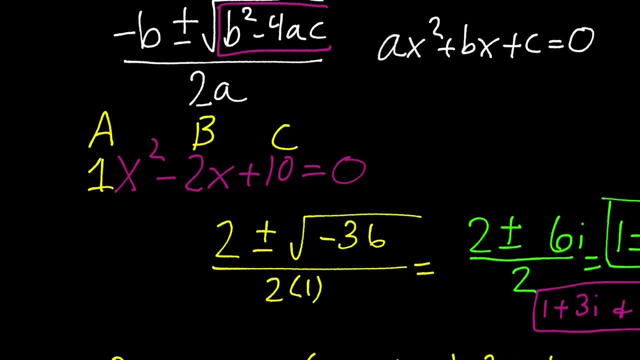 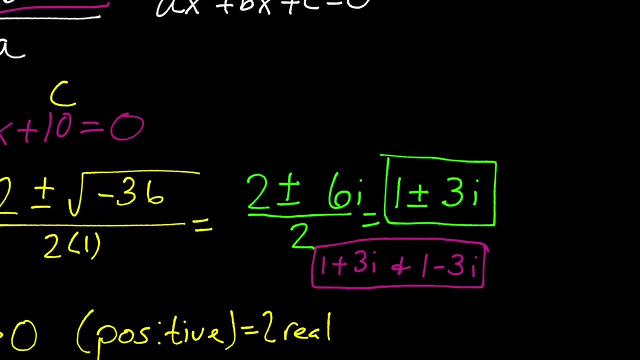 have it, We've taken this original quadratic, which ended up having non-real solutions because of a negative discriminant, and getting two non-real answers. It's a lot of work, but all it is doing is combining your knowledge of quadratic formula with imaginary numbers. 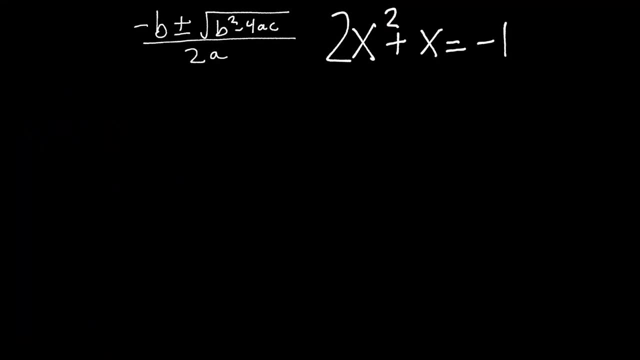 Let's try another example. For our second example, I've got 2x squared plus x equals negative 1, and we're going to use the quadratic equation to help us find our imaginary roots. Now, one thing that you hopefully notice right away is that our equation we are going to work with, 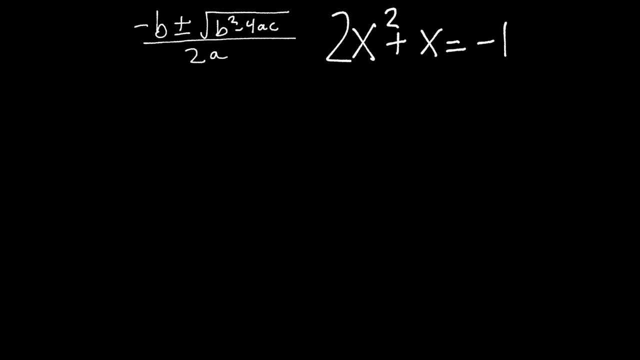 is not in the quadratic form, because it is not equal to 0. It's equal to negative 1.. So we have to add 1 to both sides so that these cancel out and become 0, and our actual equation we're going to work with is: 2x squared plus x plus 1 equals 0.. 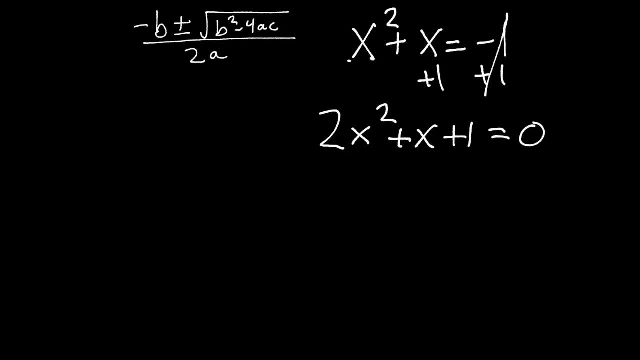 So I'm going to add 1 to both sides. So I'm going to add 1 to both sides, And until we do that we can't use the quadratic formula. But now that we have, I can get rid of this. 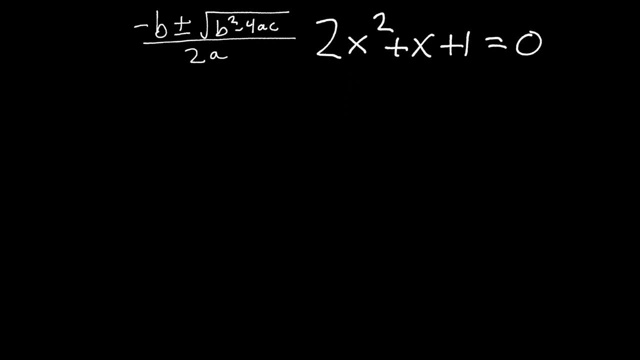 I can move this up a little bit. so it's out of our way And let's get going by first finding the discriminant. Discriminant, remember, is the stuff underneath the radical. And to make things simpler, remember A is in front of the squared term. 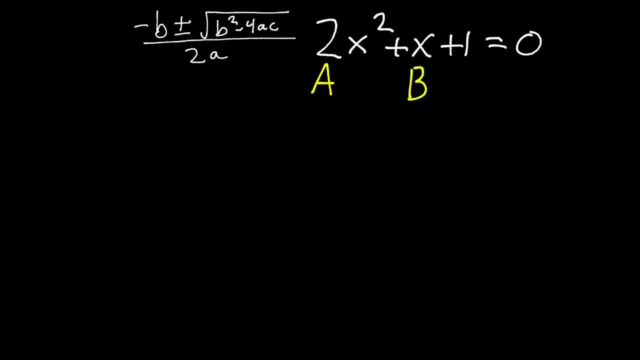 B is in front of the, B is in front of the variable, without the squared term, And C is the constant at the end. So for our discriminant here, B is going to be 1.. So I've got 1 squared minus 4 times A, which is 2, times C, which is 1,. 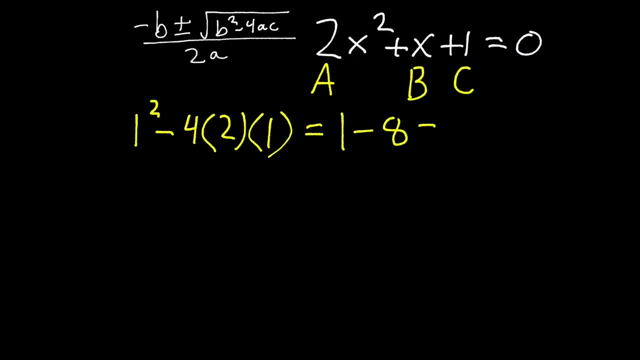 which becomes 1 minus 8, which is negative 7. Our discriminant is negative again. so therefore we have to add 1 to both sides And we have to do two non-real answers. So let's put everything into the full quadratic equation. 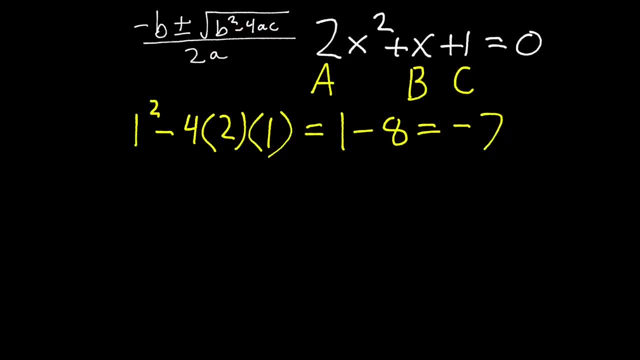 Except, remember you don't got to do this part again because you know it's negative 7.. I'll erase some of the stuff I've got here. So, creating the full quadratic equation, I've got the opposite of B, so negative 1, plus or minus the square root of 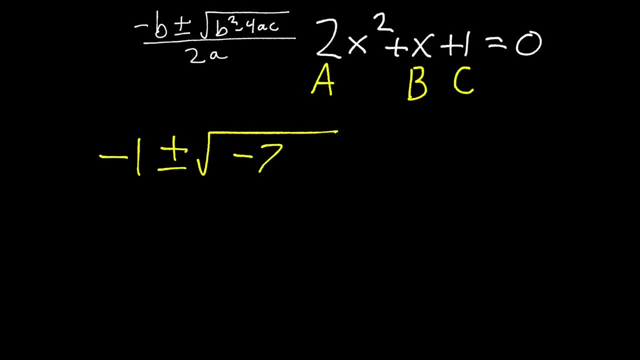 B squared minus 4AC, which we saw was negative 7, all over 2 times 2.. And we can simplify this. We get negative 1 plus or minus the square root of negative 7, all over 4.. And then we've got to deal with this square root of negative 7,. 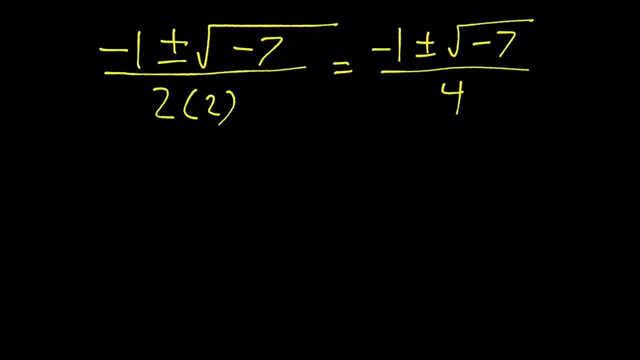 because we cannot leave it in that form. So remember: the square root of negative 7 is the same thing as the square root of negative 1 times the square root of 7.. Now we've got our imaginary term here, because the square root of negative 1 is i.